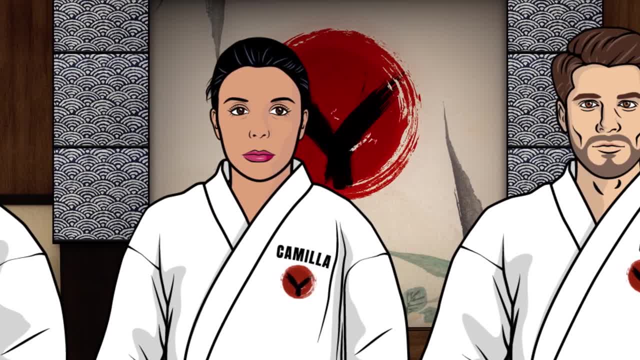 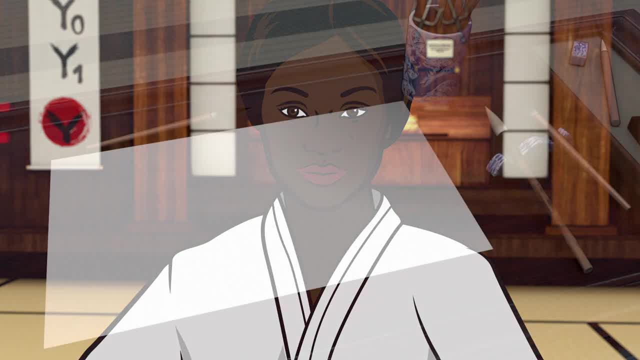 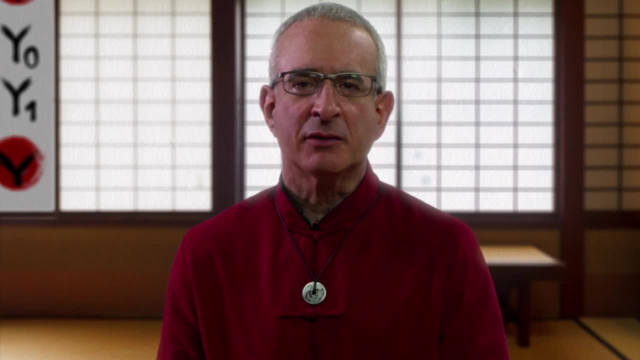 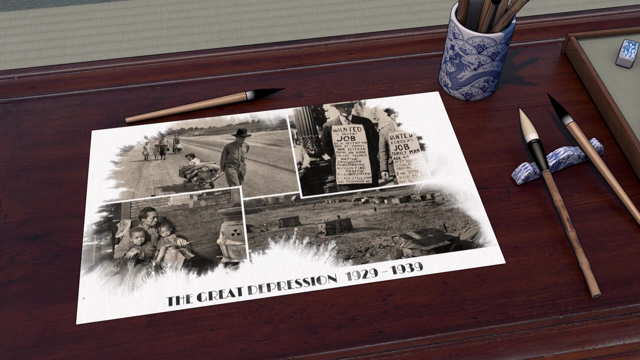 or DD- DD for short. Let's see how DD can help us understand one of the most important economic events in US history. Look back with me now at the Great Depression, the worst economic catastrophe our country has ever known. Unemployment hit 25% in 1933, a level not seen before or since. 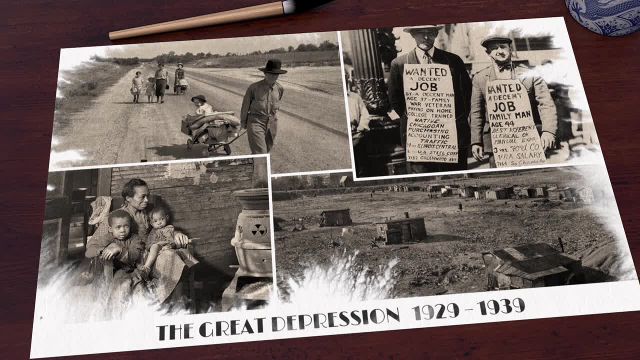 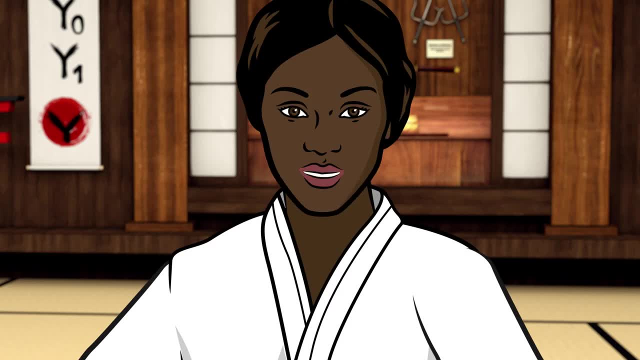 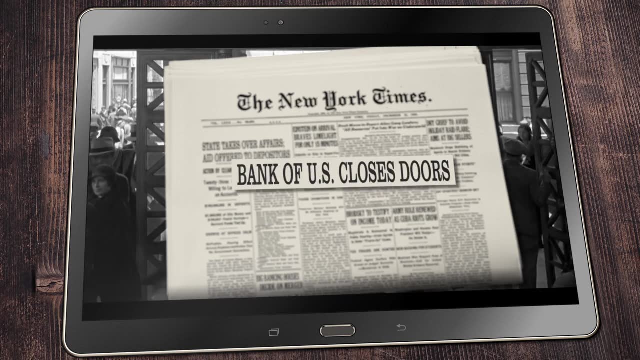 Millions lost their homes or their land. Suicides spiked hungry families relied on soup kitchens and bread lines to keep from starving. Economists argue fiercely over the causes of the Great Depression. Most agree, however, that a key piece of the puzzle is an epidemic of bank failures. 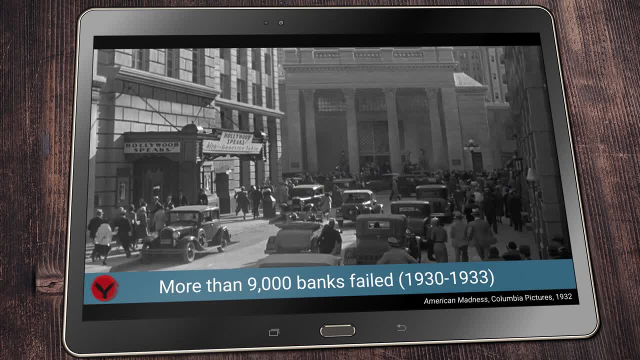 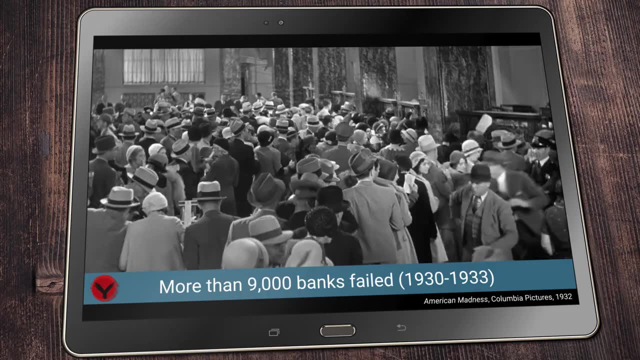 This was before deposit insurance. So if your bank went bankrupt, your savings disappeared with it Going to your account. Yes, sir, I'm going to my account. I wouldn't leave a nickel in this bank. Faced with a banking crisis, the central bank has a choice. 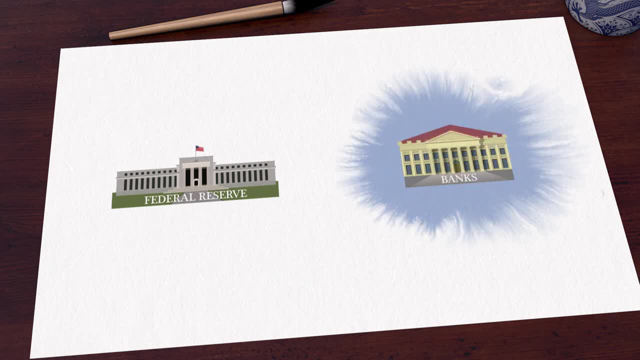 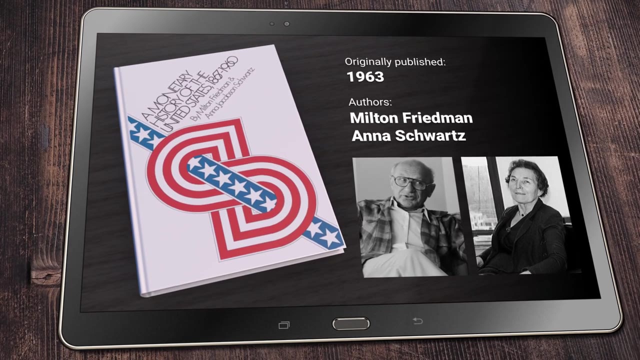 Lend freely to troubled banks or stand aside and refuse to lend. Lending freely to banks in trouble is called easy money. Refusing to lend is called tight money. Monetarist masters Milton Friedman and Anna Schwartz famously called the Great Depression the Great Contraction. 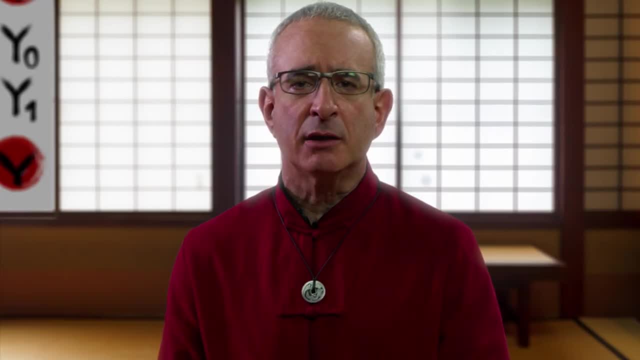 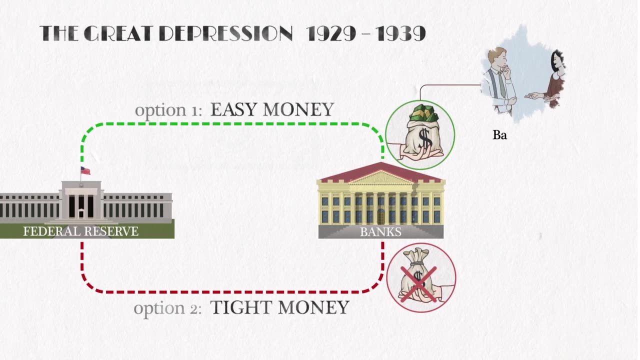 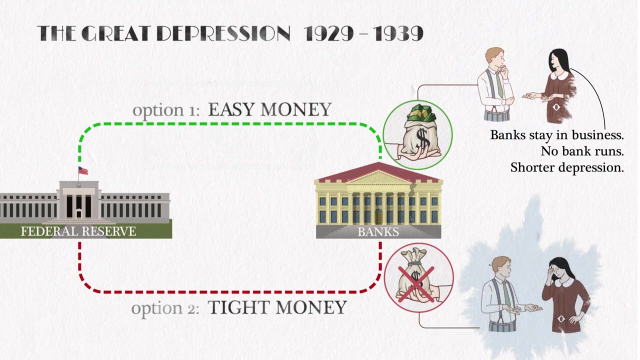 accusing the Federal Reserve of inflicting a misguided policy of tight money on the nation's teetering financial institutions. They argued that easy money would have kept many banks in business, shortening the Great Depression. But others disagree If banks are insolvent because of unwise lending decisions. 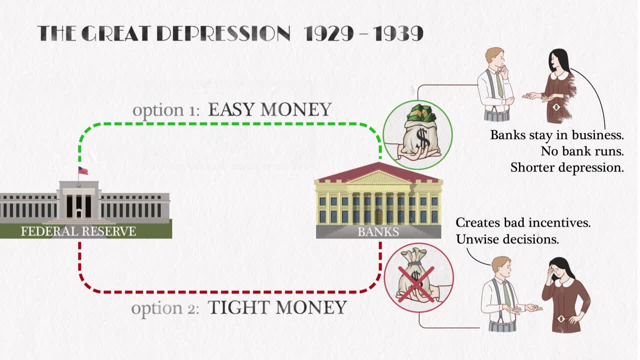 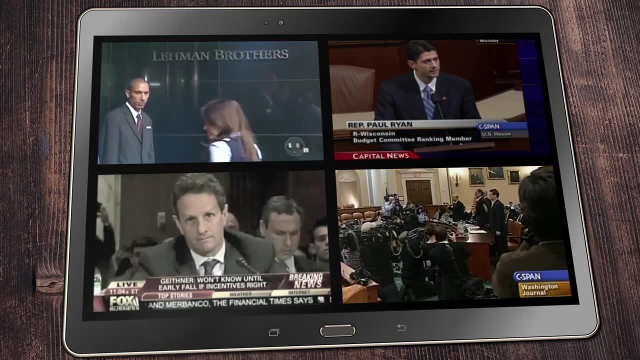 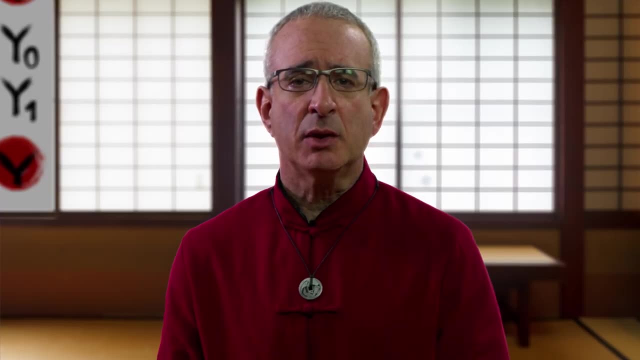 then bailouts just encourage more foolishness. Economists call this problem moral hazard. The debate over bailouts and moral hazard continues today. Should financial behemoth Lehman Brothers have been allowed to fail on the eve of the Great Recession? In an ideal world, we'd answer this question by applying different Fed policies to randomly selected regions. 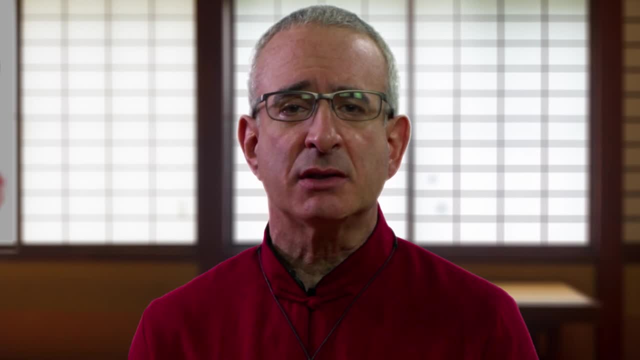 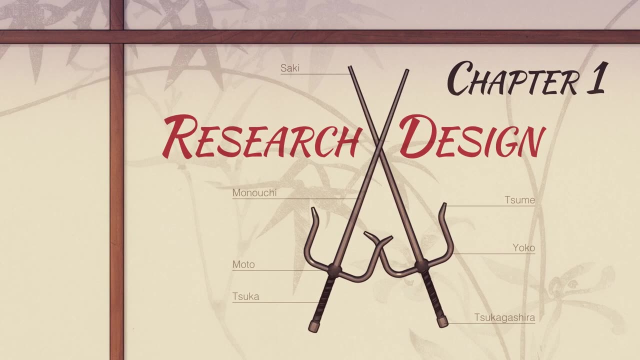 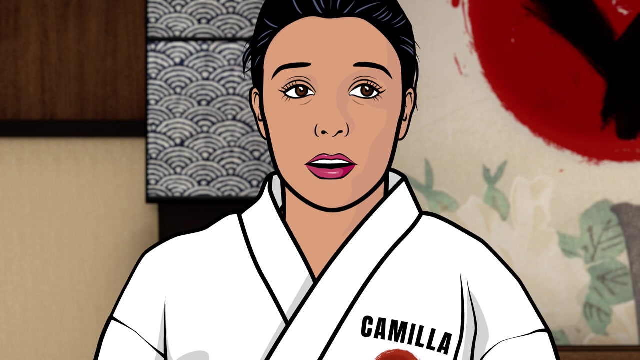 But we can still learn a lot by using differences in differences to compare trends across areas with different monetary policies. How is that even possible? Don't the same Fed policies apply to all banks in the US? Yeah, Good question. The Federal Reserve System is divided into 12 districts. 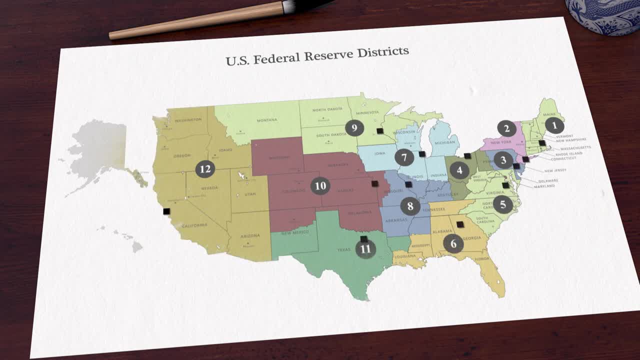 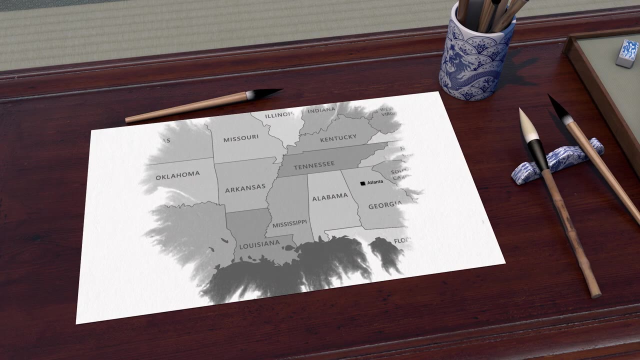 Each headed by a regional bank. Today, Fed policy is set at the national level, But in the 1930s regional Feds could do pretty much as they liked Interesting- And here's what's so awesome about that. In 1930, the Atlanta Fed running the 6th district followed an easy money policy. 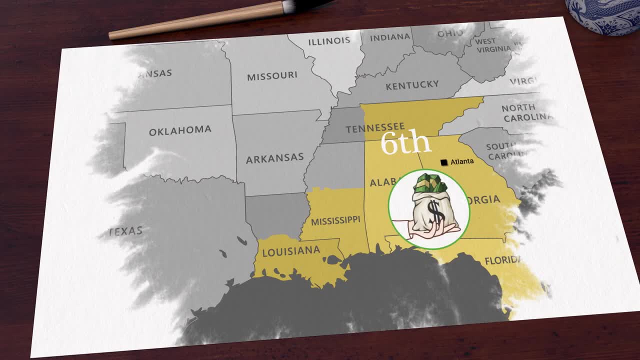 sending wheelbarrows of cash to rescue insolvent institutions. The St Louis Fed running the 8th district followed a tight money policy. Let fail the foolish, they said in St Louis, And so a natural experiment in monetary policy was born. 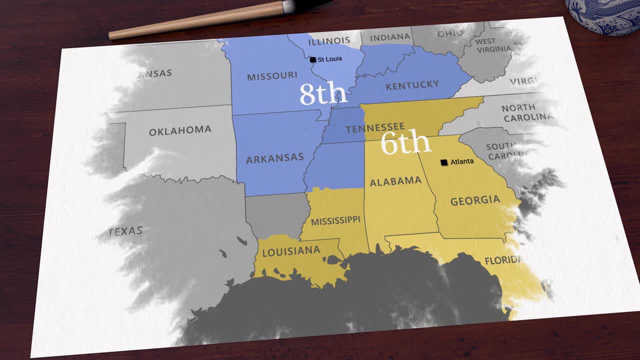 Even better. this is a within-state experiment. The border between the 6th and the 8th districts runs smack through the middle of Mississippi, So Northern Mississippi had tight money while Southern Mississippi had easy money, But under the same state laws and banking regulations in both. 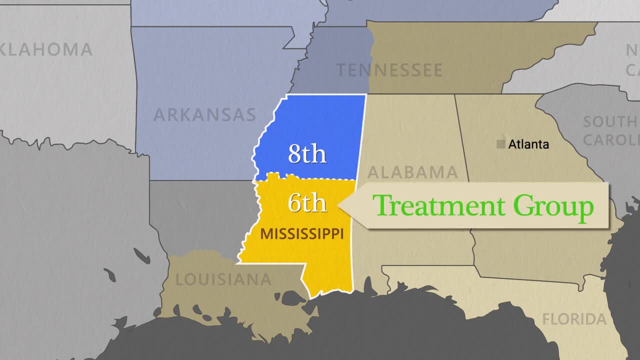 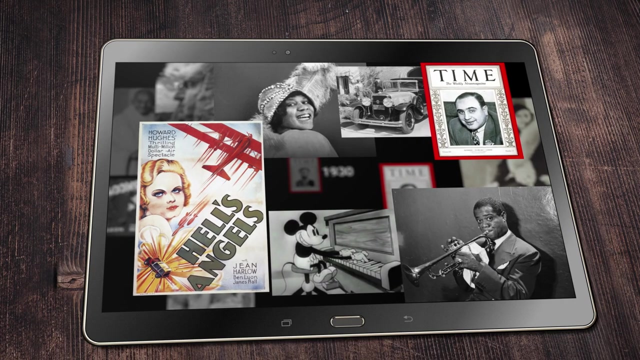 The Treatment Group is the District 6 part of Mississippi Which had access to easy money during the crisis. The Control Group is the District 8 part of Mississippi Which had tight money during the crisis. The key year in our natural experiment was 1930.. 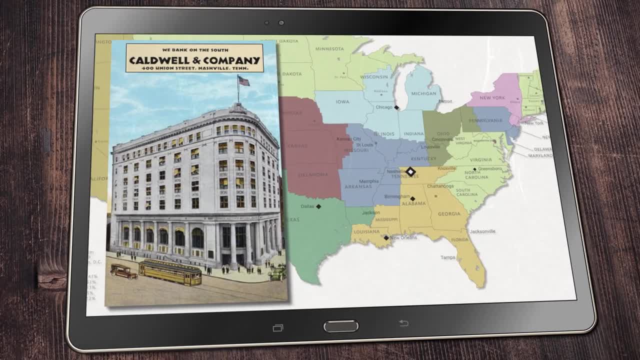 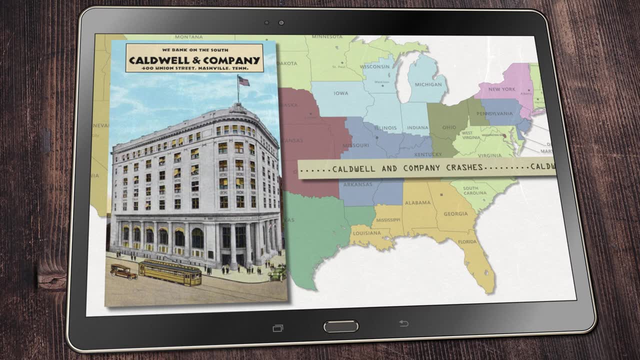 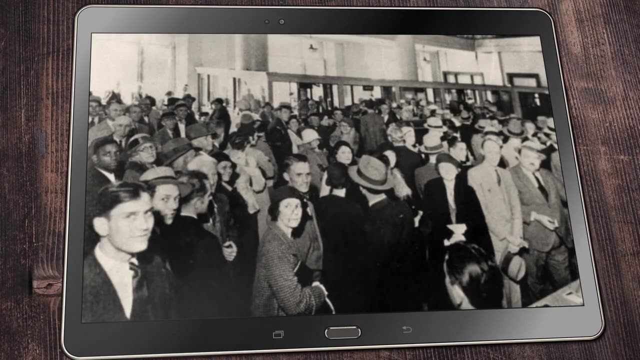 Caldwell and Company, a massive financial empire in the South, came crashing down. Banking is a business built on confidence and trust. The Caldwell meltdown caused a panic That led to a widespread bank run. All at once, depositors wanted their money back. 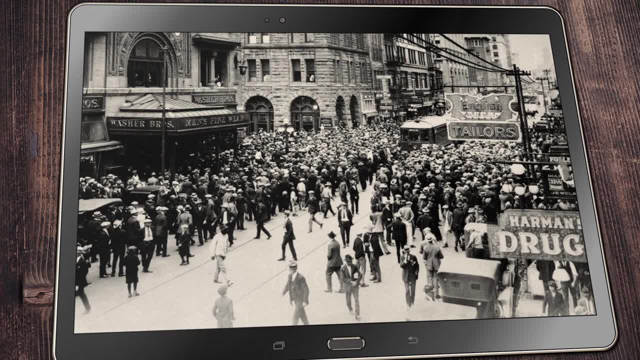 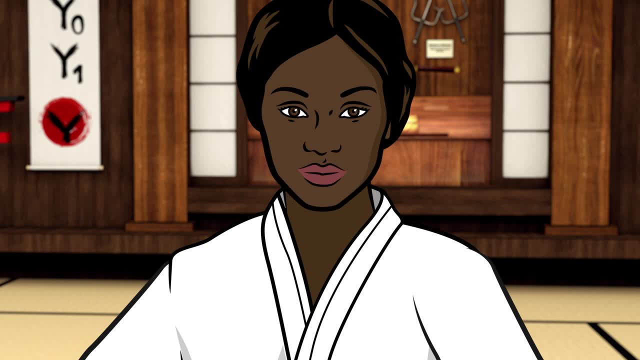 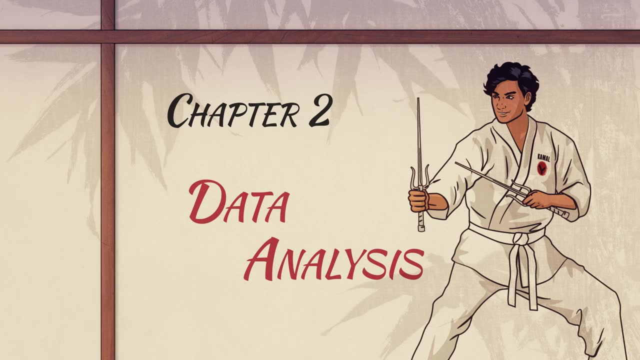 Causing banks to go bankrupt and shut their doors. We'll use differences in differences to measure the effect of contrasting monetary policies in response to the Caldwell crisis. This figure plots the number of banks in Mississippi by year, for the 8th and 6th districts. Let's start in 1929, a year before the Caldwell crash. There are 169 banks open in the 8th and 141 banks open in the 6th. Over the next year, we see a similar handful of banks fail in both districts. 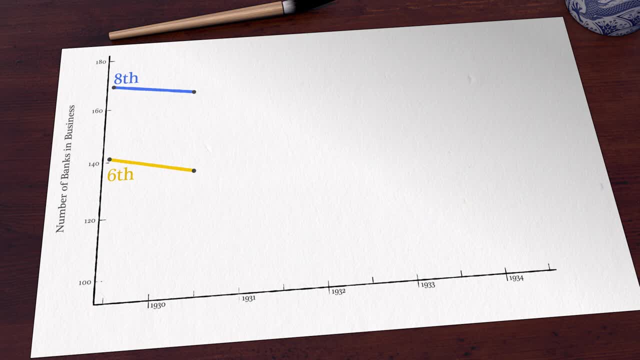 The change in the number of banks in operation is remarkably similar. That's what parallel trends look like In November 1930, Caldwell crashes And the panic begins. Banks fail frequently in the 8th district, which had tight money, But the decline is slower in the 6th district, which had easy money. 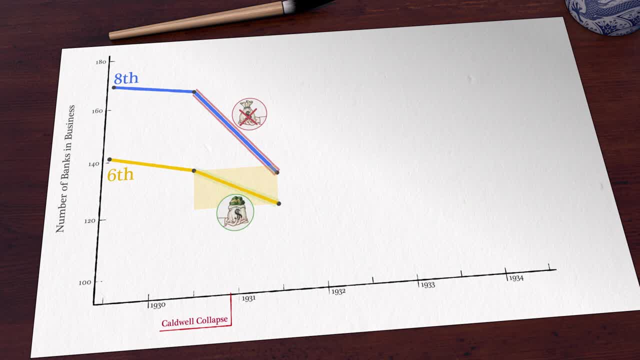 The diverging trends in this period might be attributable to easy versus tight money. In July of 1931, the 8th district abandons tight money. So now both districts are easy. Parallel trends are restored In a counterfactual world where the 6th district follows a tight money policy. what might have happened? 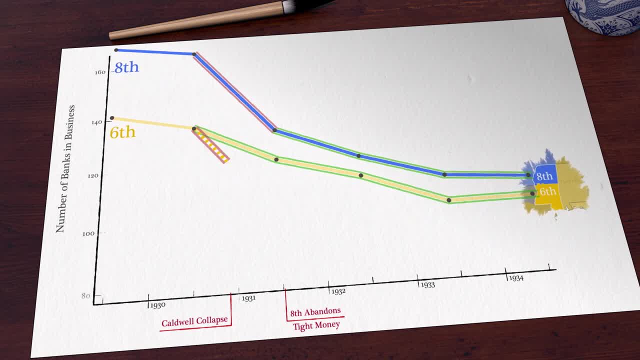 If we extrapolate the trend of the 8th district to the 6th, it would look like this. So the treatment effect of easy money is how much the 6th district deviated from the path implied by the 8th district trend. How many banks did the easy money treatment save? This table reports data for the treatment group in the first row and data for the control group in the second row. The first column shows the number of banks in business before the crisis began in 1930.. 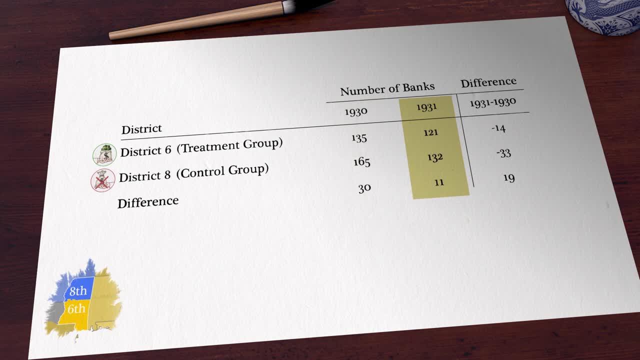 The second column shows 1931. This is the key period when each district had differing monetary policies. during the crisis, The rightmost column reports changes within the district. District 6 lost 14 banks, while District 8 lost 33.. The mathematical formula for the treatment effect is simple. 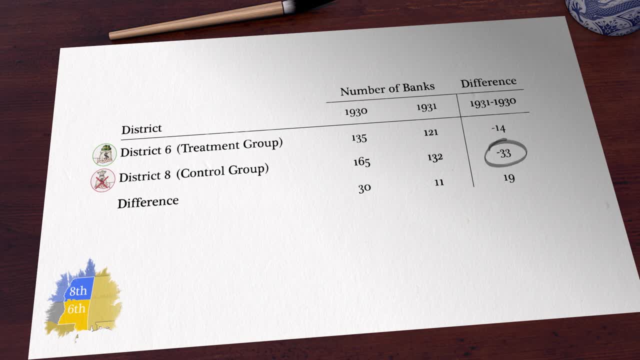 We subtract the change in banks in operation in the 8th district from the change in banks in operation in the 6th, Hence the name. differences in differences: Negative 14 minus negative 33 equals 19.. We estimate that 19 banks were saved by easy money. 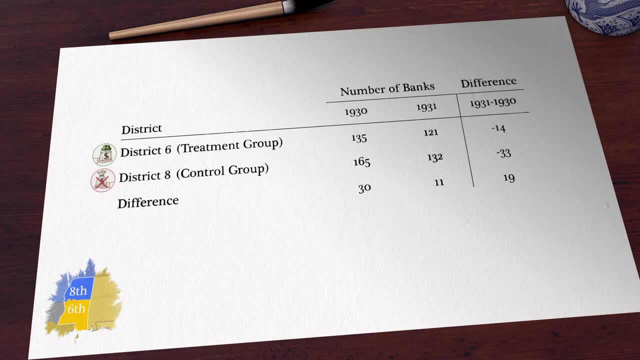 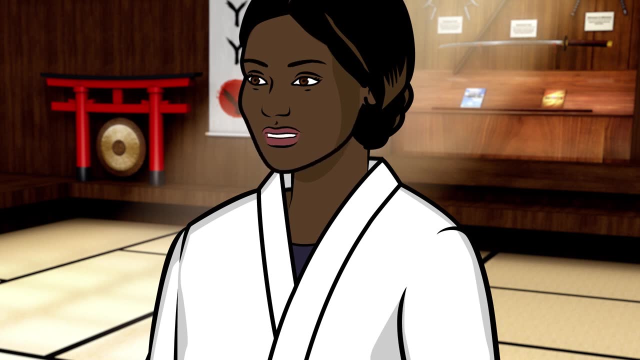 In practice, tables and figures like those shown here are the beginning rather than the end of a DD analysis. The problem of how to gauge the statistical significance of DD estimates turns out to be exceedingly tricky, and a regression is typically part of the solution. 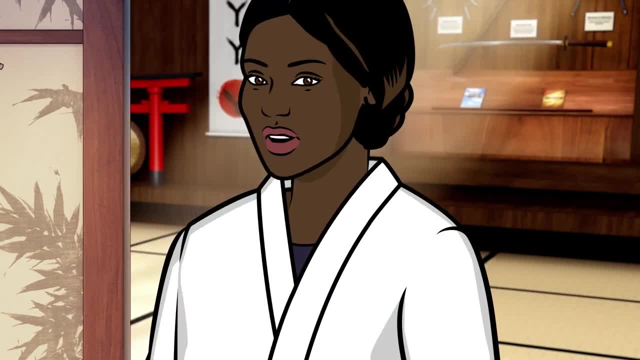 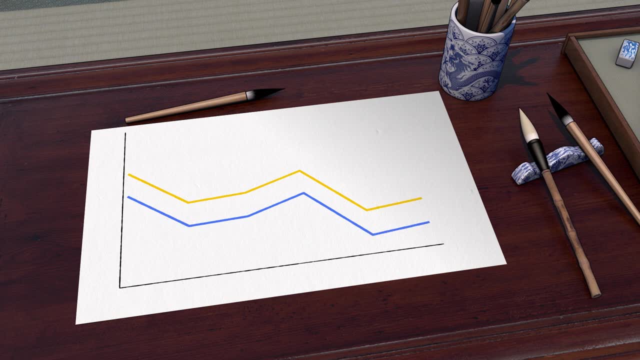 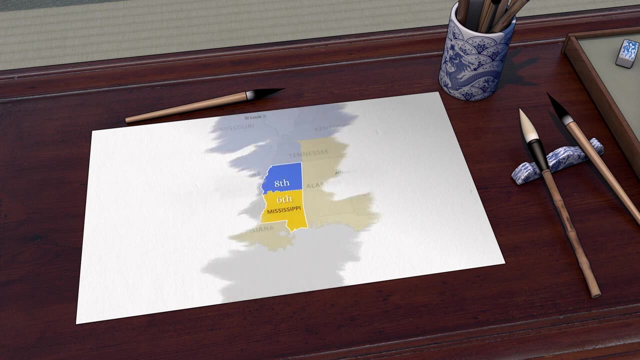 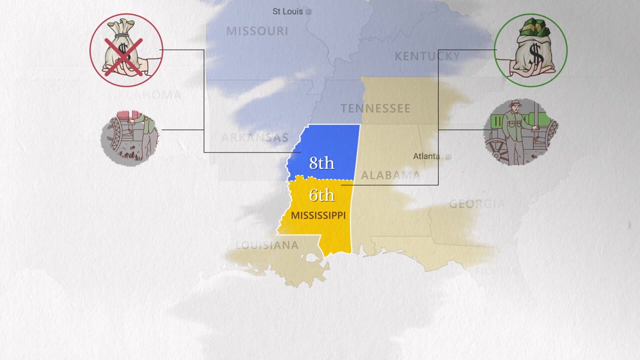 The key assumption behind a valid DD analysis is that of parallel trends. Recall the principle of Ceteris Paribus. Our ideal comparison would have the two districts experience an identical business environment, except for one factor – easy or tight money. Both districts would have identical types of customers who would go bankrupt at exactly the same rate. 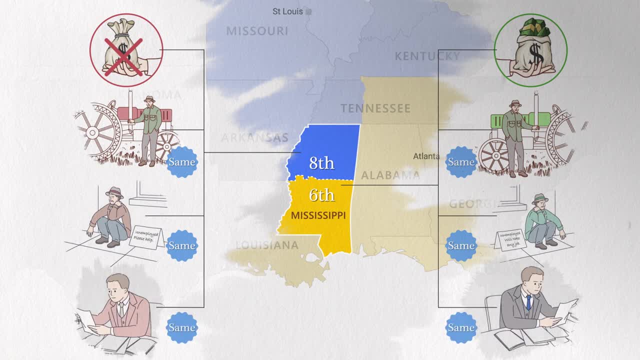 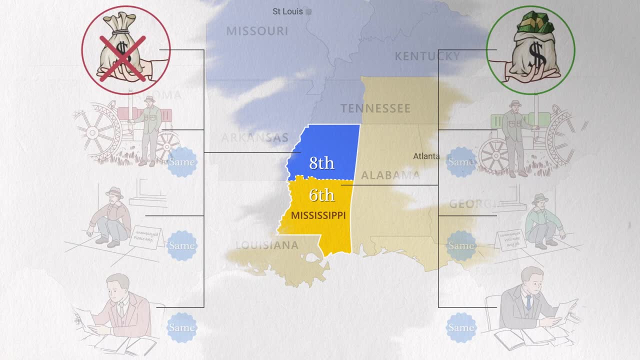 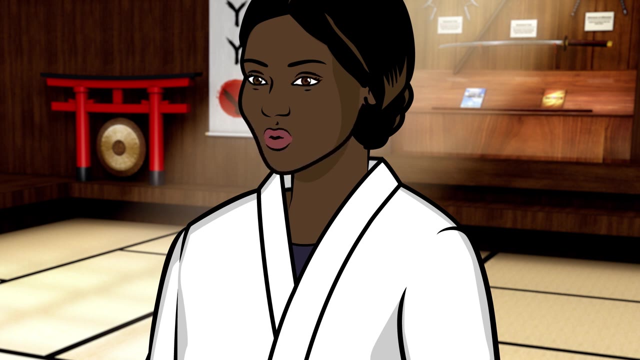 The skill of their employees would be equal, and so on. Perfect Ceteris Paribus comparisons would allow us to clearly see the causal effect of different Fed policies. In this case that's not possible, But the idea of parallel trends is based on a similar concept. 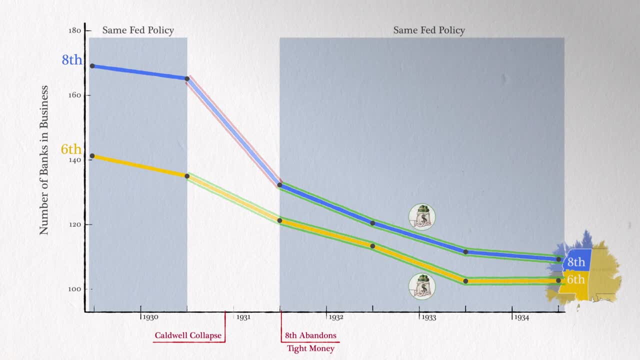 If we see that the two regions experience similar trends in the number of banks over time in the absence of treatment, we can assume they are good comparisons. We see that the two districts move in parallel both before the crisis and after, when they have the same Fed policy. 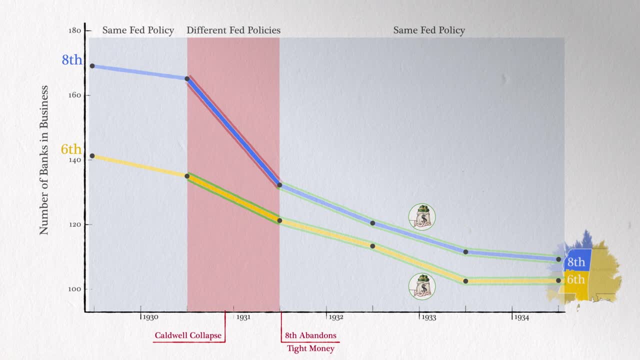 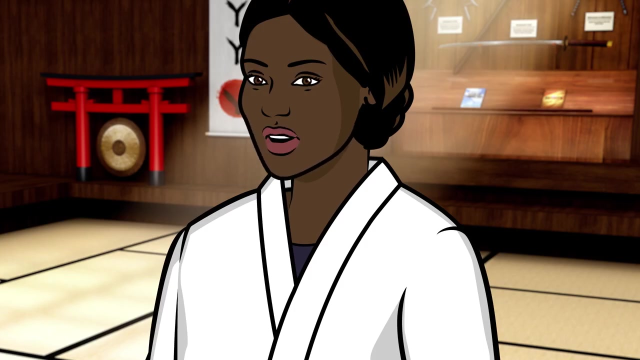 The only time the districts behave differently is when the Fed policy is different. In view of this, Fed policy is a likely cause of diverging trends from 1930 to 1931. But we should also check for other changes unique to northern Mississippi. 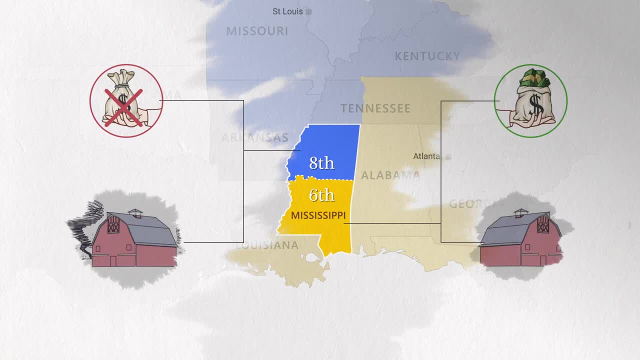 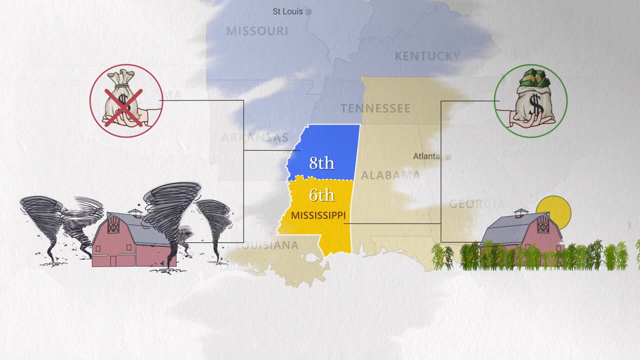 What do you mean? Imagine that bad tornadoes hit northern but not southern Mississippi in 1930. These tornadoes devastate farms, causing farmers to default on loans, which drives their banks out of business. Then the 6th and 8th districts would differ in not one, but two ways – Fed policy and weather. 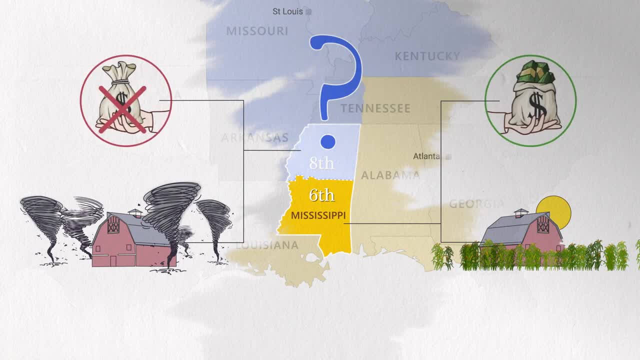 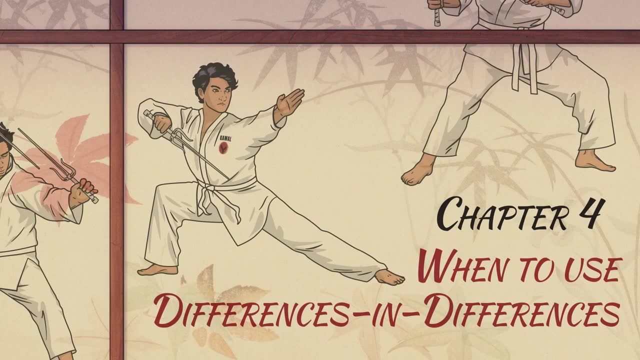 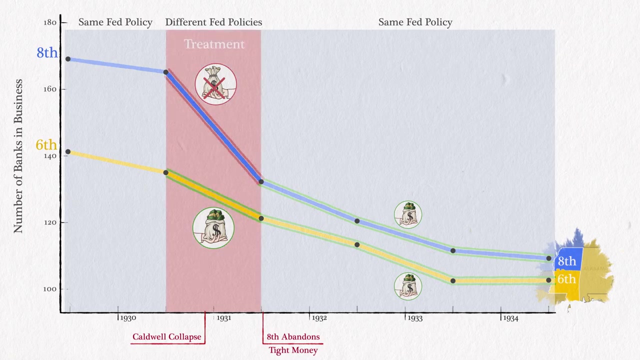 And we'd have trouble identifying Fed policy as the causal factor behind increased bank failures in the 8th. This is not Paris DD. credibility lives or dies with the claim that the only reason northern Mississippi was special in 1930 is differing regional Fed policy. 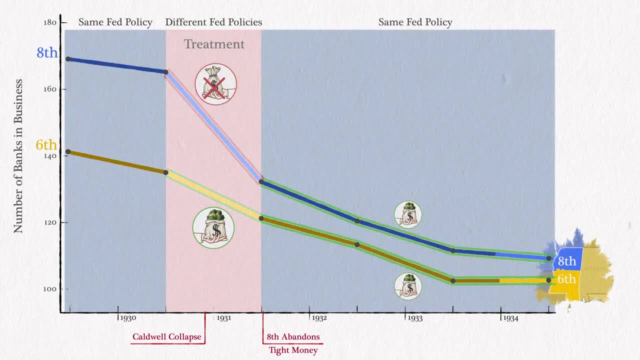 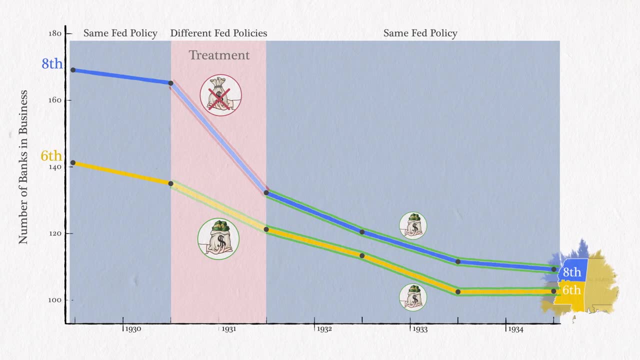 We're in DD heaven with strong visual evidence of parallel trends. In general, the first step in evaluating whether to use DD is usually this type of visual confirmation of parallel trends outside of the period when we're in the middle of a crisis. This is outside of the period when we expect to see a treatment effect. 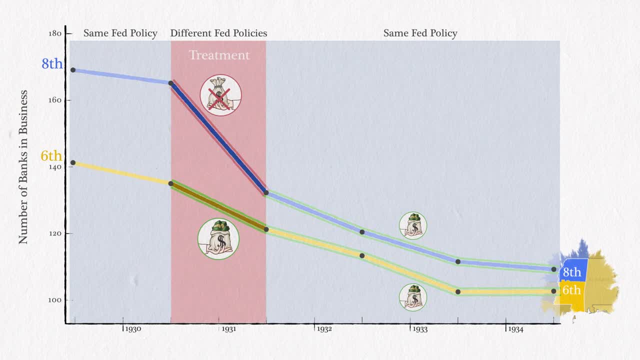 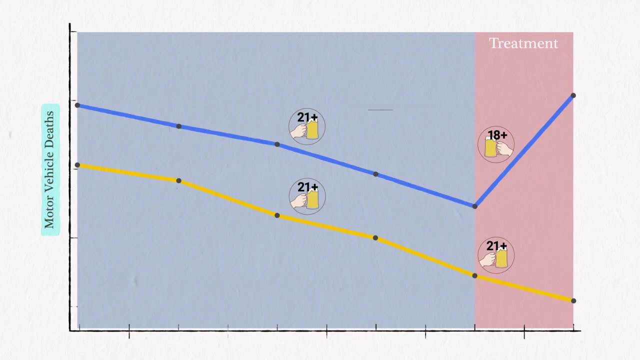 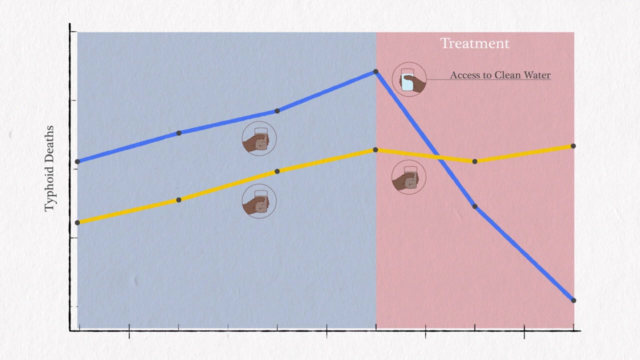 The treatment in our example is easy money in the face of bank failures. Metrics masters use DD to explore effects of many policies like the minimum legal drinking age, and environmental changes like access to clean water. In our next video, we'll see an example of how regression is used to implement a DD approach. 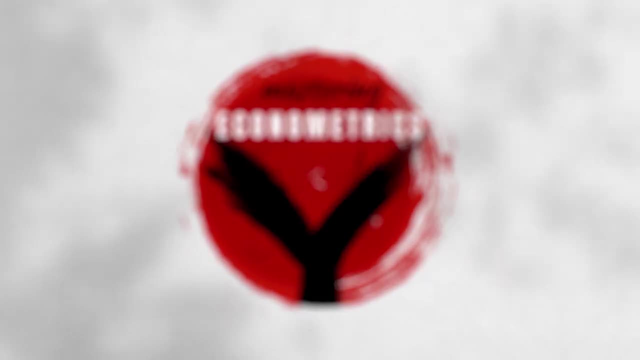 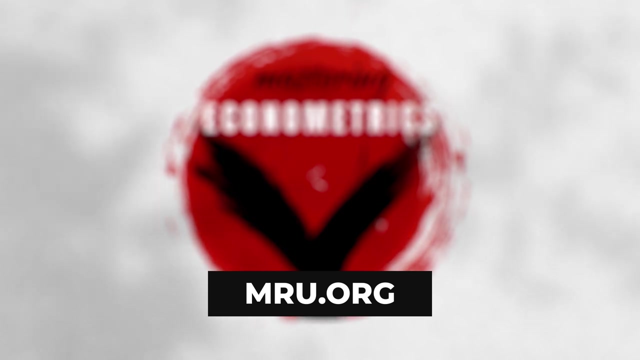 Are you a teacher? Click to explore ways to use these videos in class. If you're a learner, make sure this video sticks by taking a few quick practice questions. Or if you're ready, click for the next video. You can also check out MRU's website for more courses, teacher resources and more. 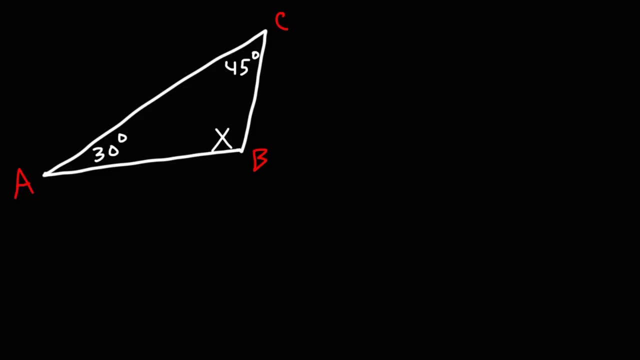 In this video, we're going to talk about how to calculate the missing angle of a triangle. So we're going to start with some simple examples, and then we're going to escalate to harder problems. 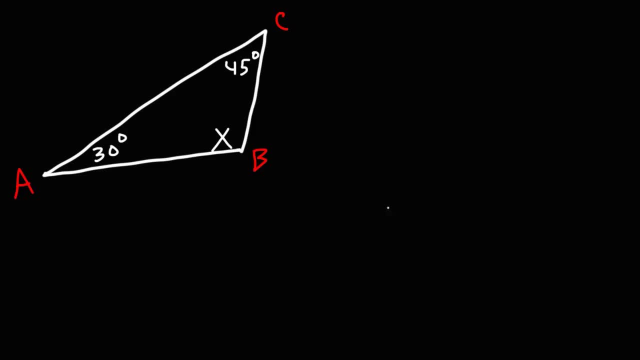 So let's start with this problem. We need to calculate the angle X or angle B. How can we do so? Well, we need to know that the three angles of a triangle add up to 180 degrees. 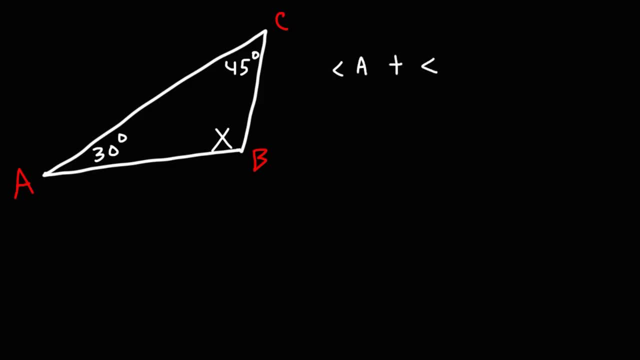 So angle A plus angle B plus angle C adds up to 180. Angle A is 30 degrees. Angle B, that's X. Angle C is 45. So if we add 30 plus 45, that will give us 75. Now, in order to calculate the value of X, 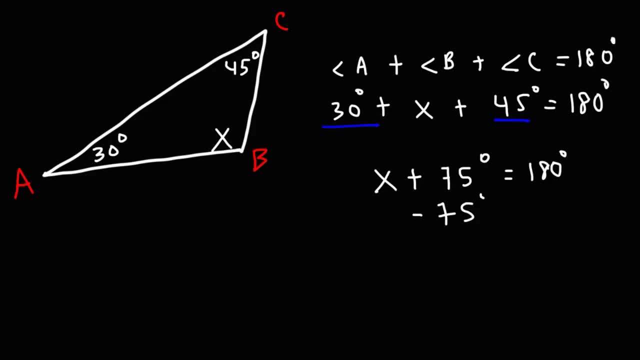 We need to get X by itself on one side of the equation. So we need to subtract both sides by 75 degrees. So X is 180 minus 75, or 105. 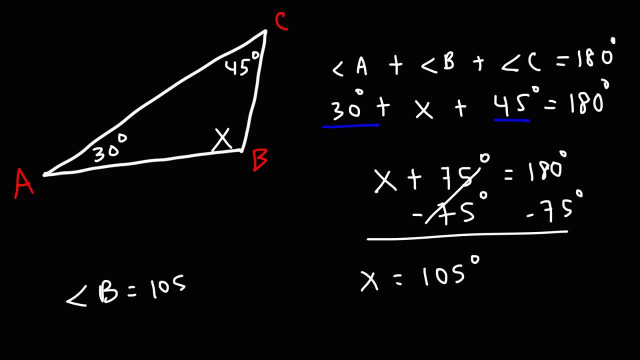 So the measure of angle B is 105 degrees. So that's the answer for this problem. 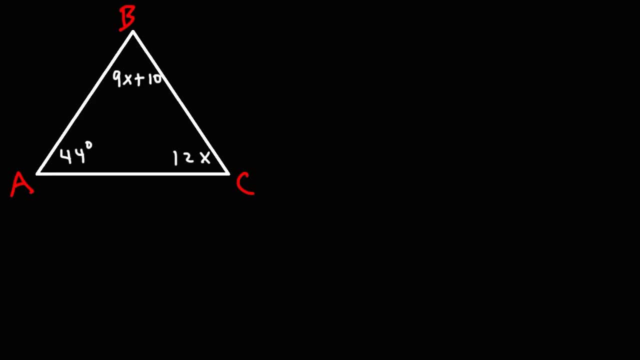 So now let's move on to our next problem. We're given that angle A is 75 degrees. Angle B is 44 degrees. 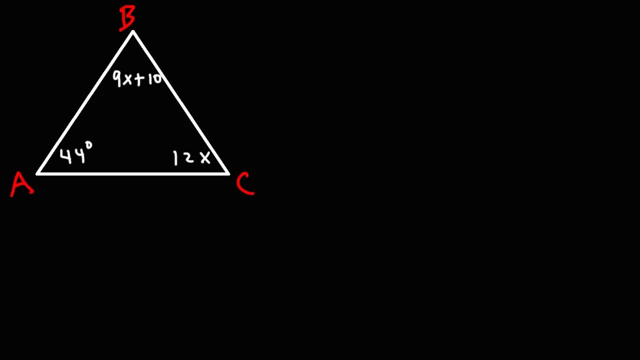 Angle B is equal to 9X plus 10. And angle C is equal to 12X. 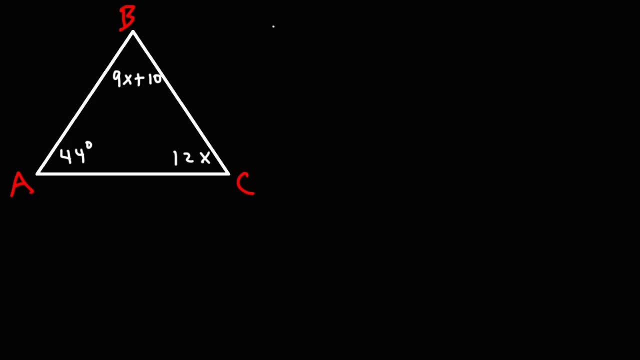 So take a minute and try this problem. So we can start with the same formula. 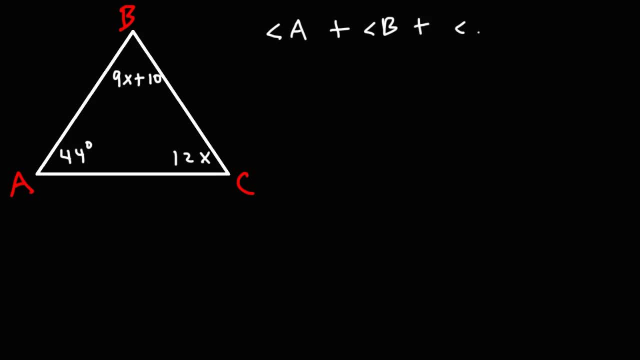 All three angles of any triangle must add to 180. 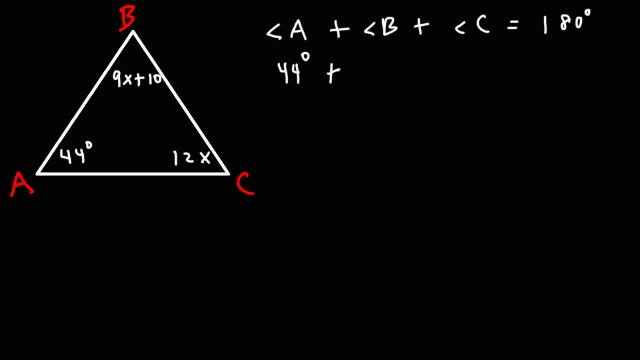 Angle A is 44. Angle B is 9X plus 10. And angle C is 12X. 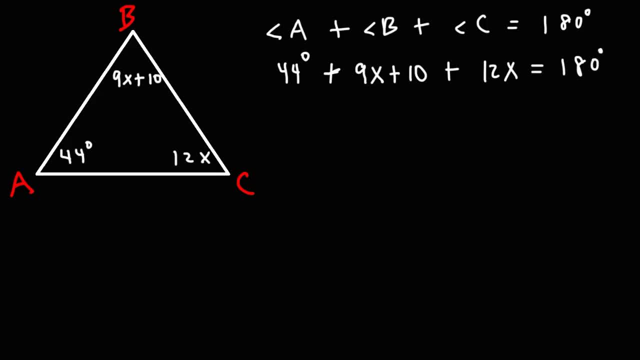 So now let's do some math.